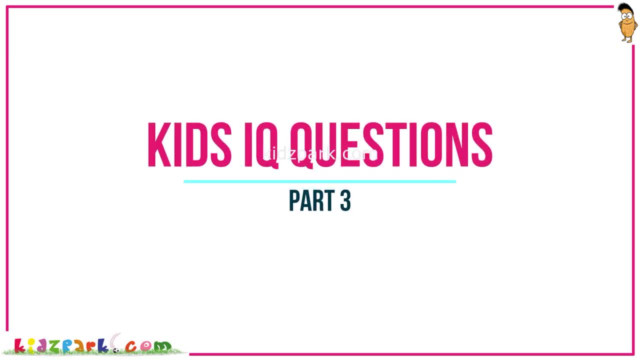 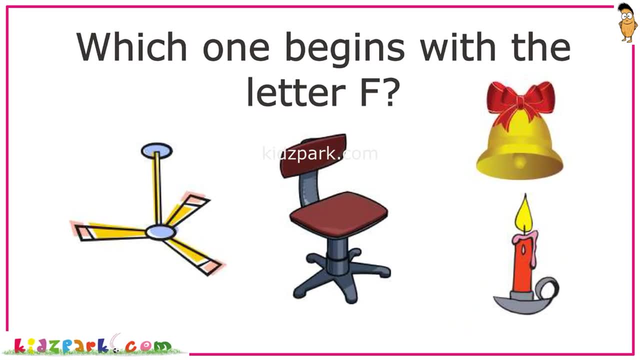 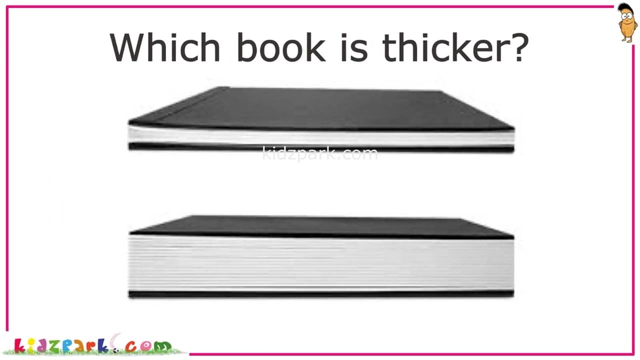 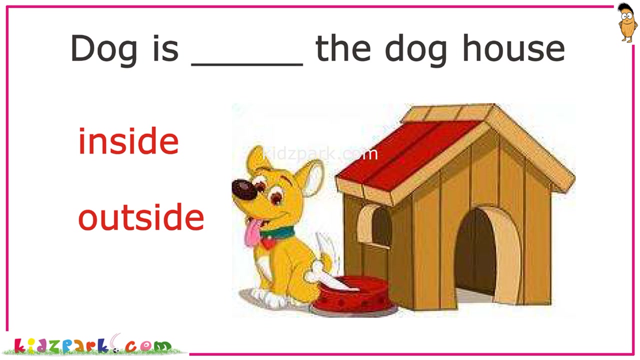 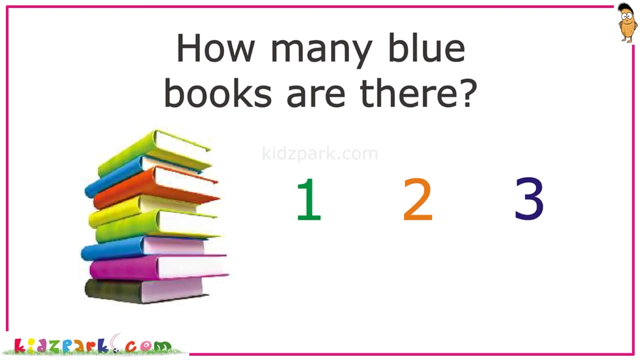 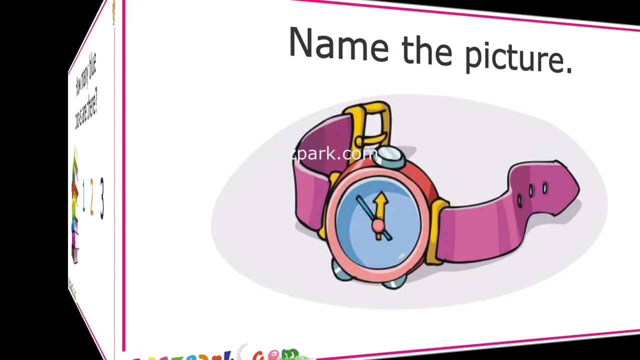 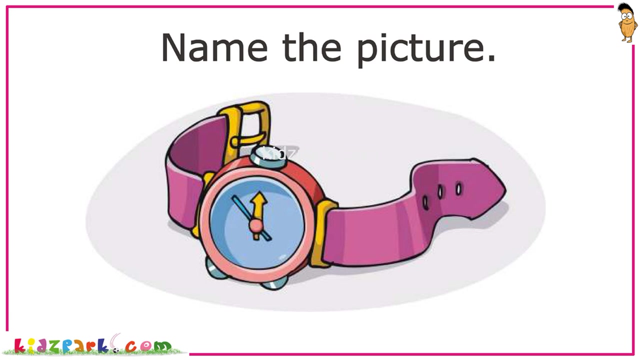 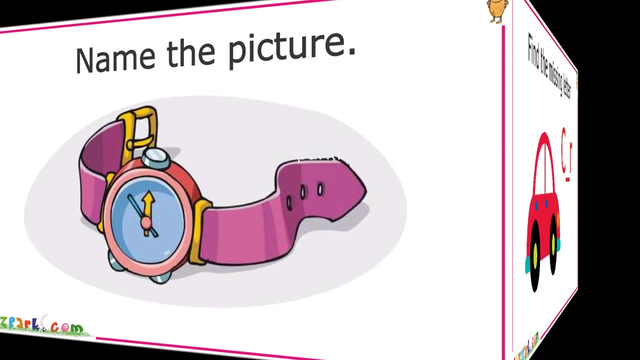 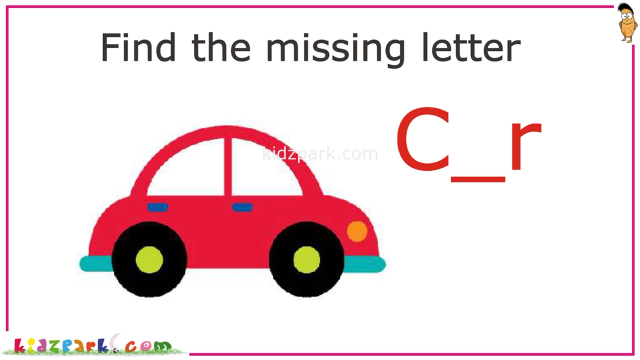 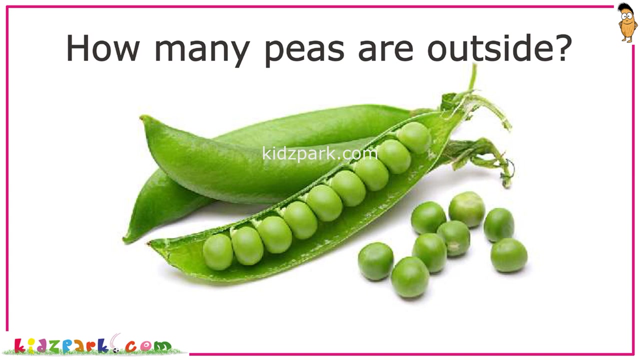 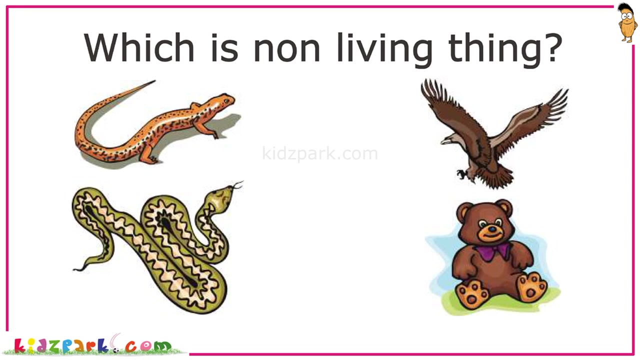 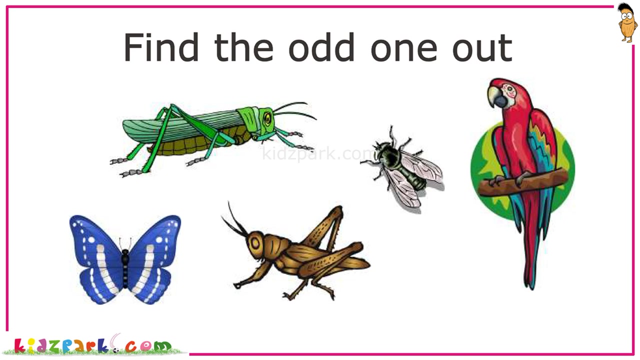 Which one begins with the letter F? Which book is thicker? Dog has dashed the doghouse. How many blue books are there? Name the picture. Find the missing letter. How many peas are outside, Which is non-living thing? Find the odd one out.